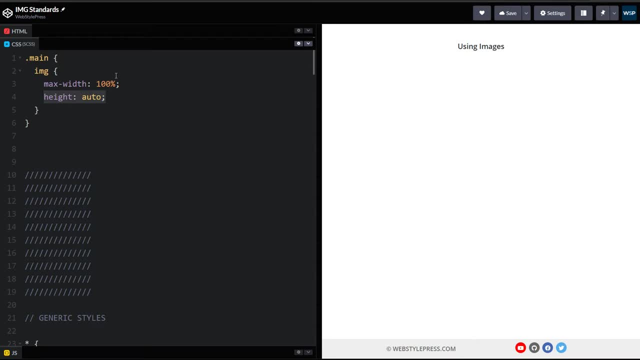 If their loading does not affect other elements on web page and if they are loaded only when needed, then you need to wait for a few seconds to load. If they are loaded only when needed, then you need to wait for a few seconds to load. If they are loaded only when needed, then you need to wait. If 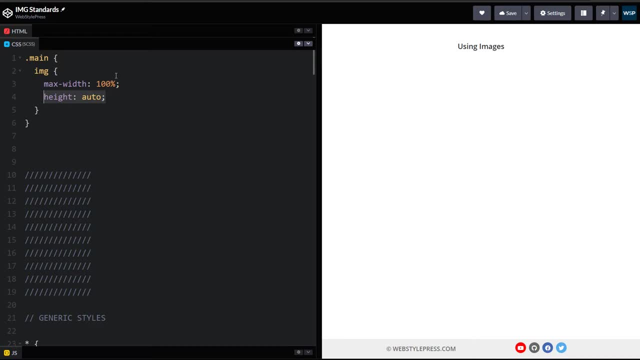 they are loaded only when needed, then you need to wait. If they are loaded only when needed, then you will make sure your website loads extremely fast. So let's improve how we use images in website. First of all, we need additional attributes in IMG tag for lazy loading and for async support. 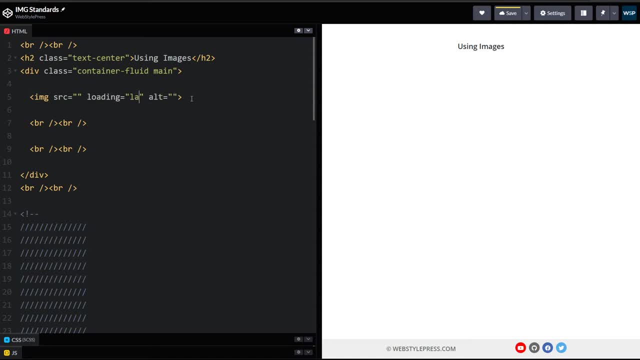 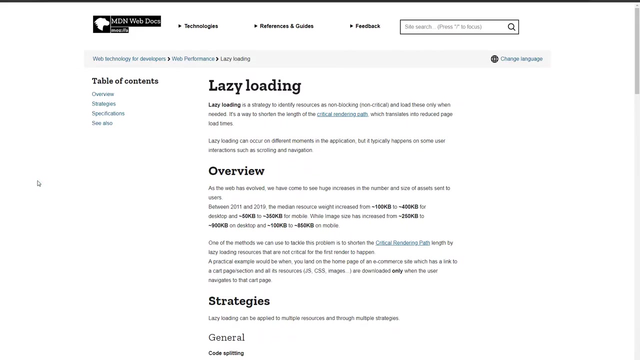 Loading lazy and then decoding async. The loading attribute specifies whether a browser should load an image immediately or to defer loading of off-screen images until the user scrolls near them. This attribute may not be supported for all browsers, but where it is supported, it will help a lot. You can read more about lazy loading at MDN web docs. 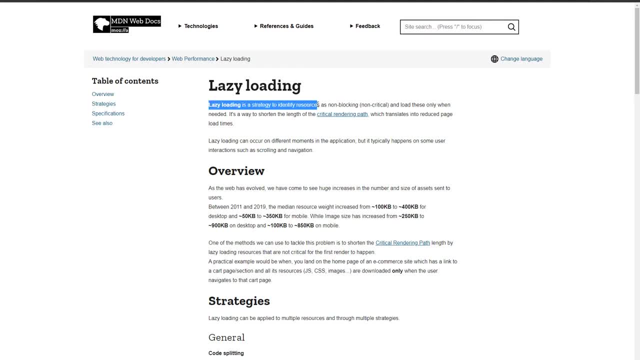 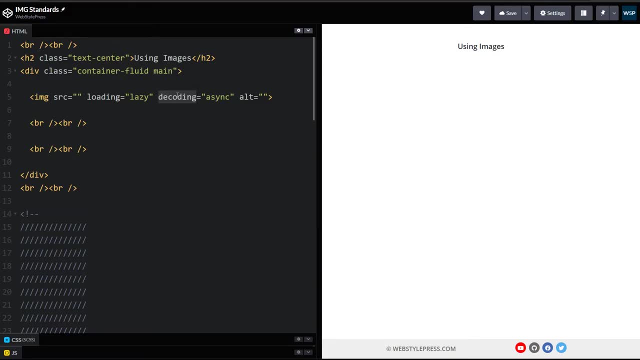 Lazy loading is a strategy to identify resources as non-blocking, non-critical, and load these only when needed. The decoding property of the image represents a hint given to the browser on how it should decode the image. Async value means to decode the image asynchronously to reduce delay in presenting other content, While images will. 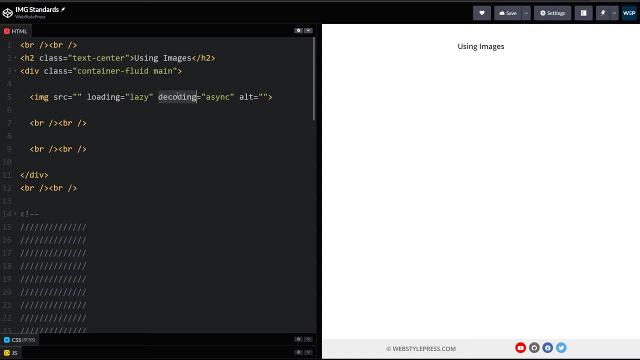 be loading other web page, content won't be affected. Do not ignore these two Attributes. make this mandatory for all images. Then we have CSS upgrade for images. I'm adding these two lines: Content visibility auto and background color: light gray. Content visibility auto will load. 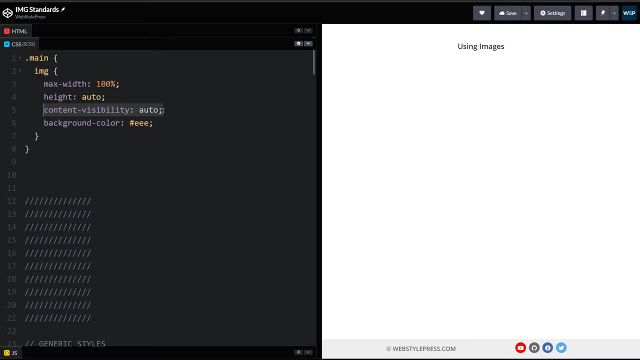 image when it is needed. We used loading lazy in image tag, but here it is CSS implementation. I will use both. We used background color for image to show background color as a placeholder. When image will be loading, a nice background color will be displaying space that image will acquire. 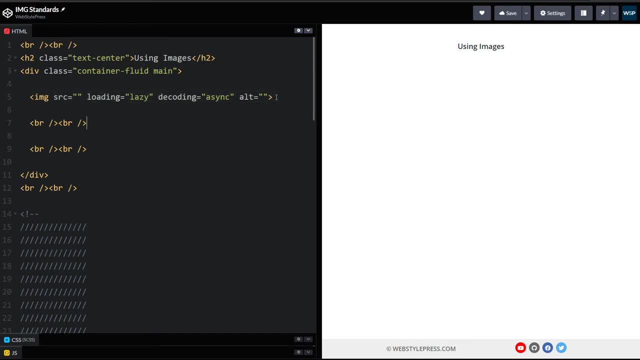 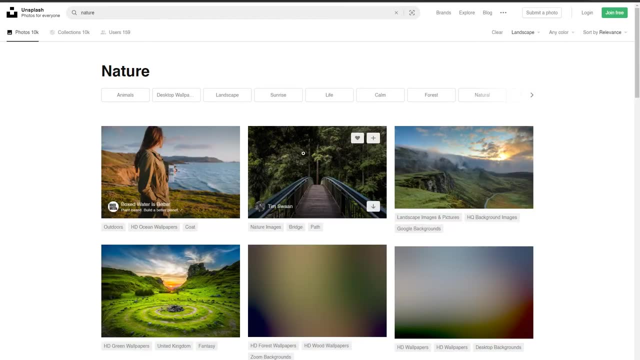 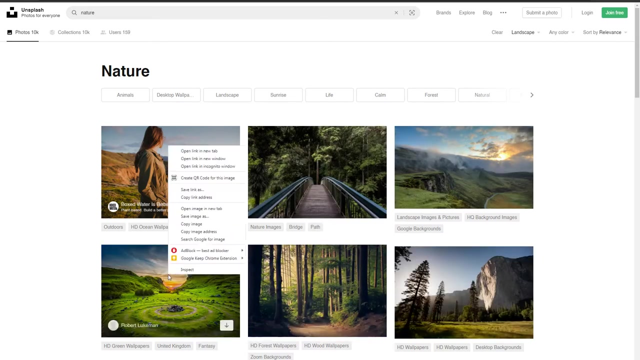 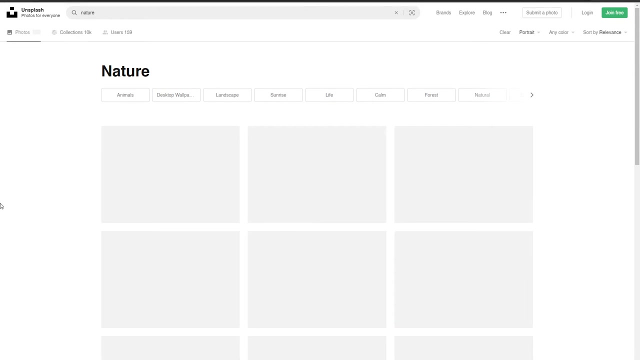 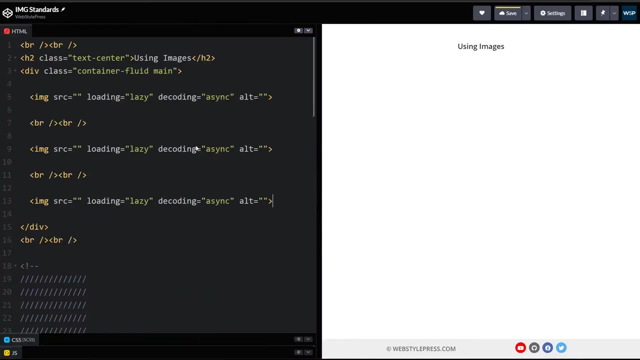 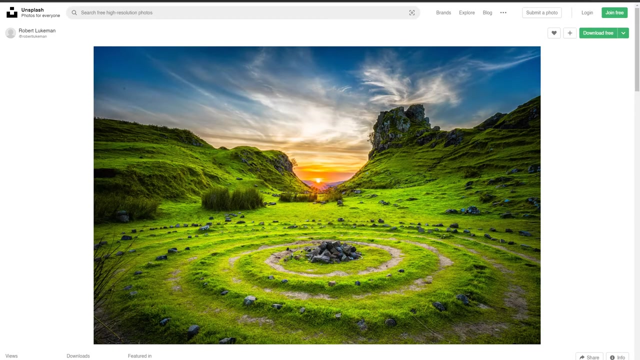 Let's add few images here. We need three images. Let's choose landscape. I will choose this image and then this one. Also, choose one portrait styled image: Copy image address In this source. here is our image Copy image address. I want you to notice gray. 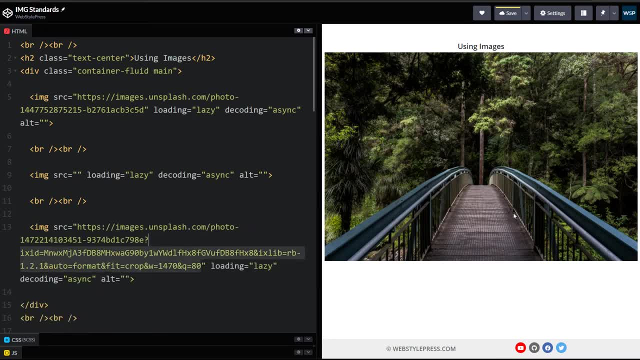 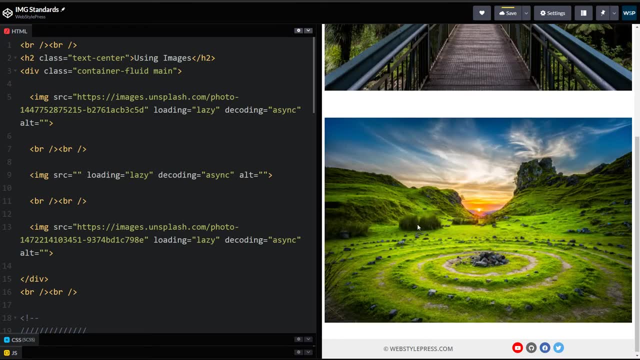 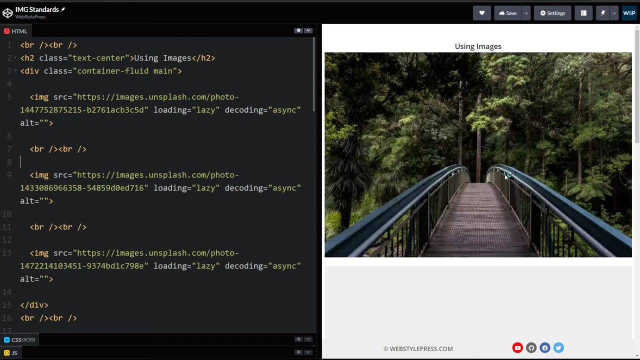 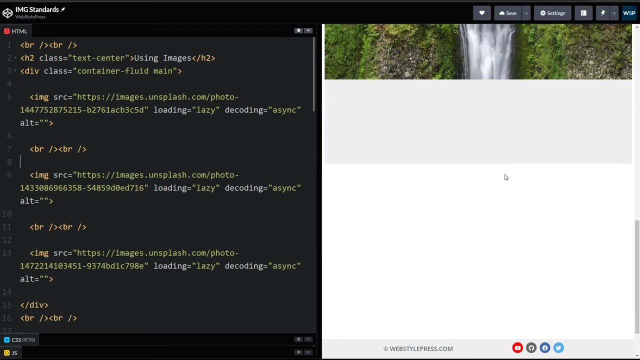 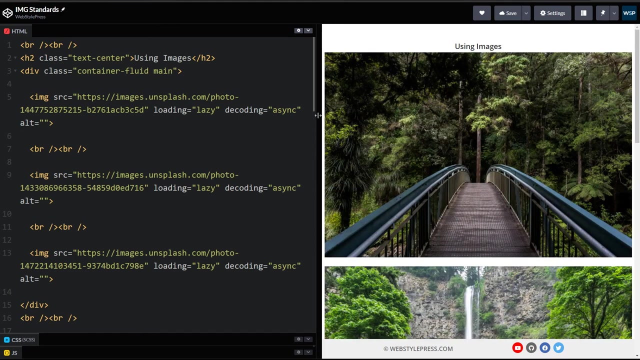 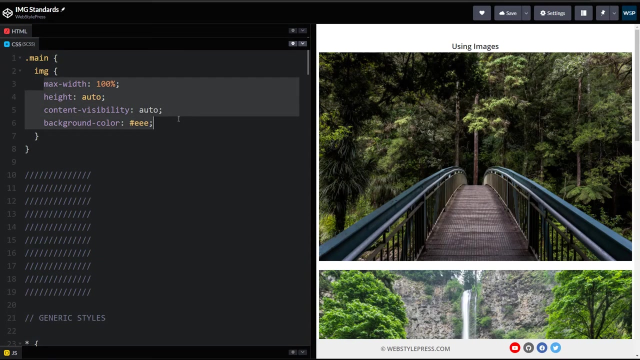 background when image will be loading. See this gray background. and this is a third image: cup image address and head. then we have content layout shift issue. you may have used Google, Pagespeed or lighthouse. they complain if content shifts during page load, for example, if you do not. 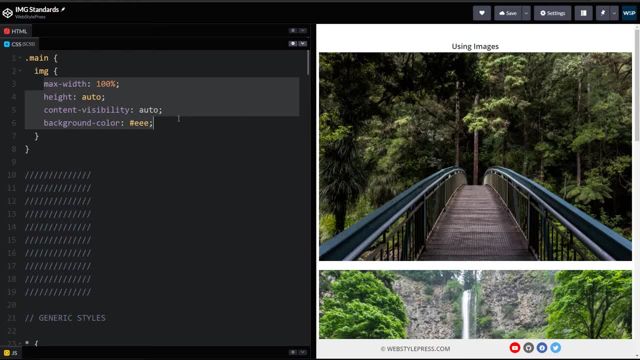 specify image width and height. nothing will be displayed during image load. when image is loaded, it will shift content placed under it. further below there will be content jump. during page load will be displayed. it will also signify that page load is currently not uploaded. so we may stitch shower page load as shown in the video after check in of page load when the image is. 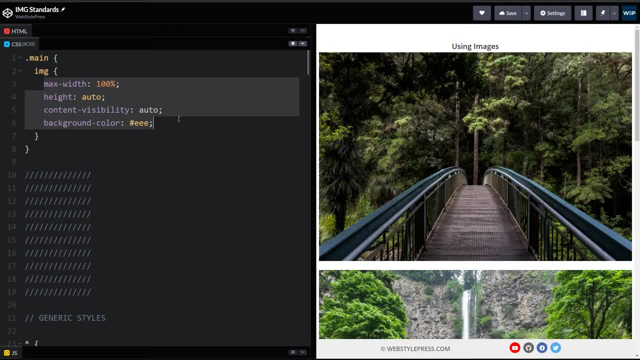 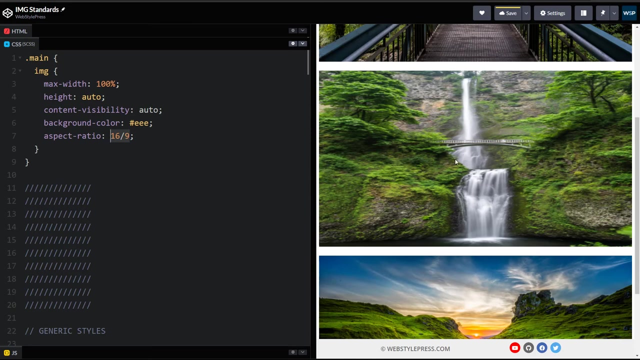 page render and page speed insight will indicate that content layout shift can be avoided if we specify image width and height or we can use aspect ratio css property, that is, aspect ratio 16 by 9. but as you can see, this image is disturbed. now aspect ratio 16 by 9 can be used for wide. 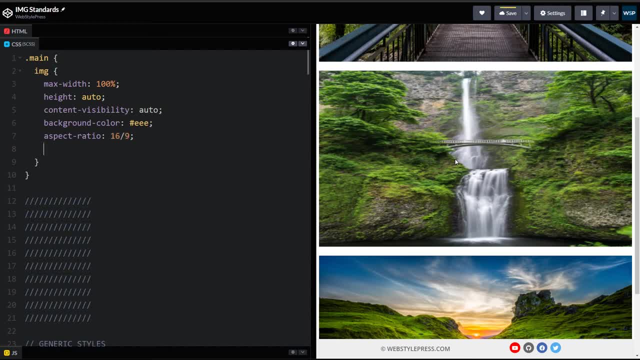 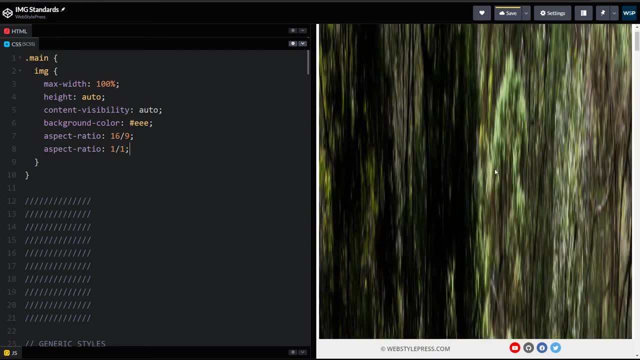 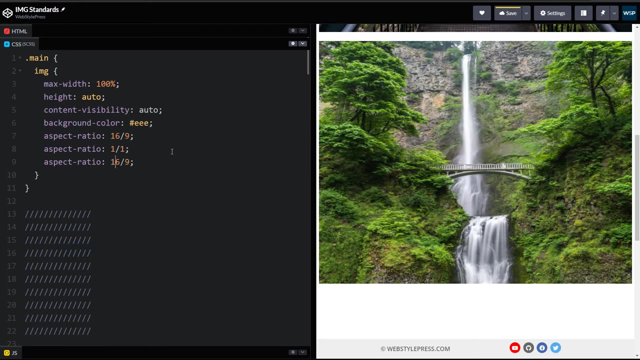 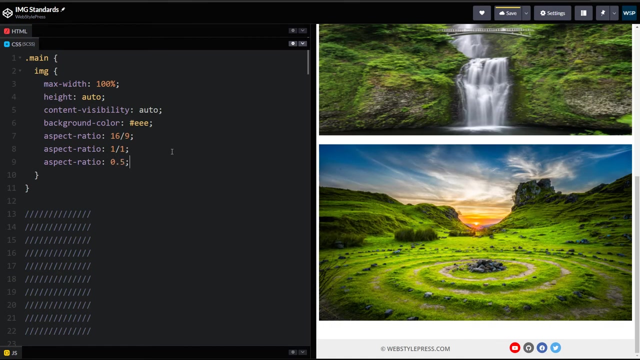 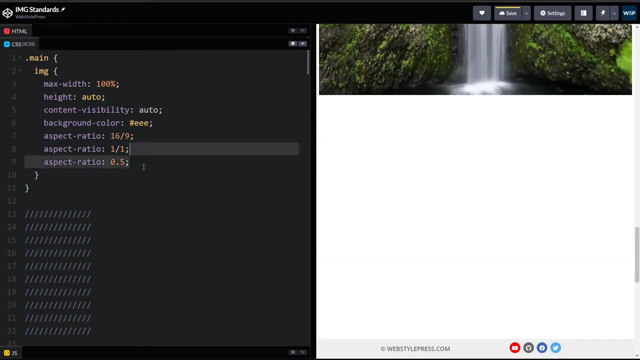 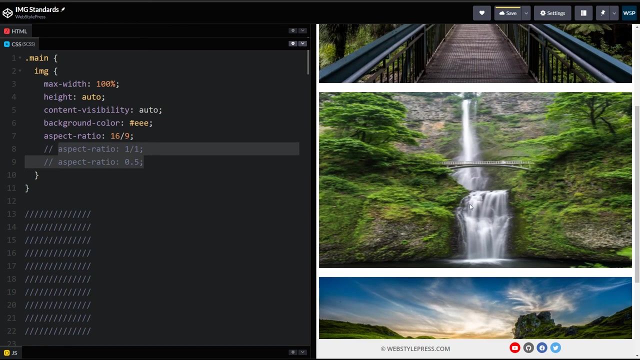 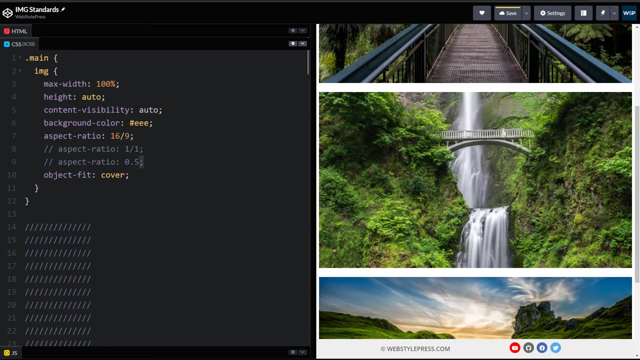 images. there are other aspect ratios as well. for example, expect ratio one by one or aspect ratio half, and this image is distorted. now, to control this unnecessarily stretch, we can use object fit cover and now the image is better. but this image was not wide. so what we can use, we can also use a spec ratio one by one for such image. 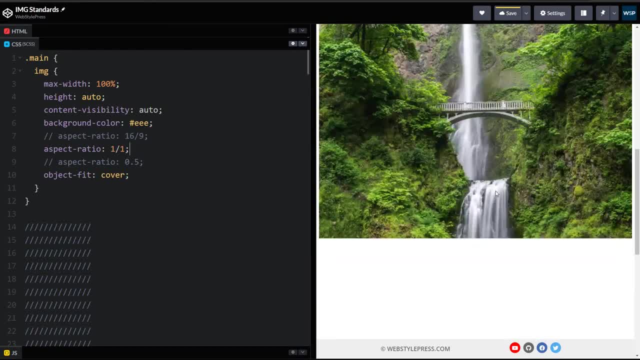 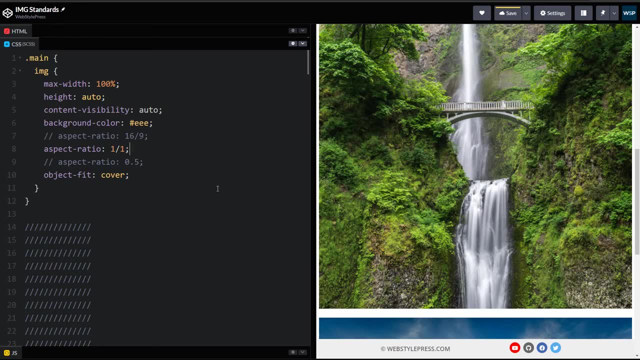 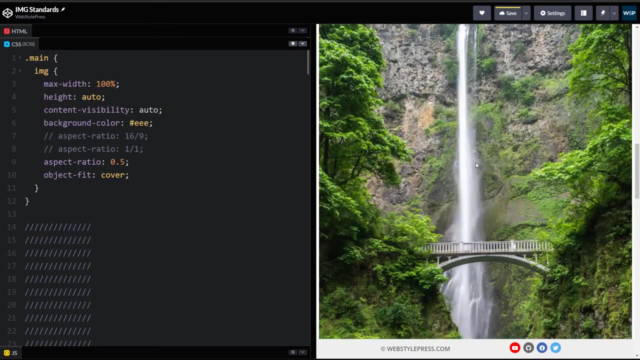 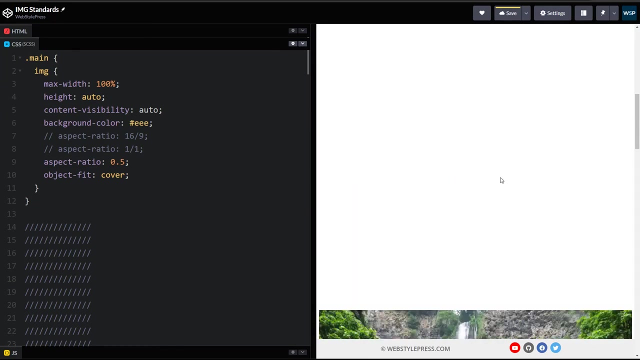 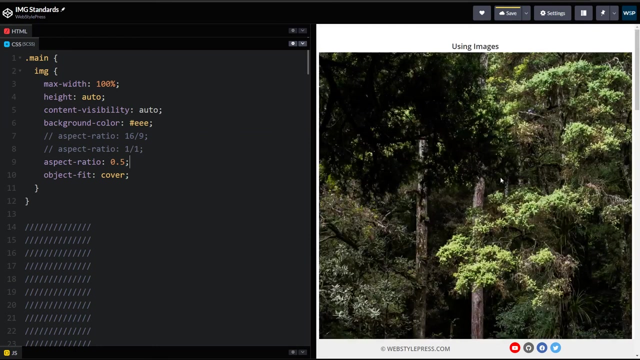 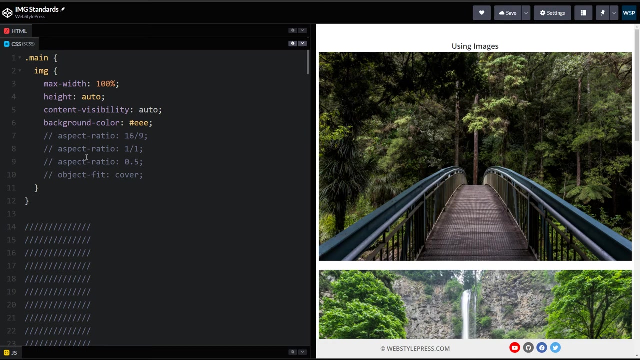 we can also use a spec ratio one by one for such image or half. now this image is all right, but other images may be disturbed. you see this was a wide image. you can add. this is a main view effect- if you find aspect ratio an object fitCON − inner side not appropriate for all images. 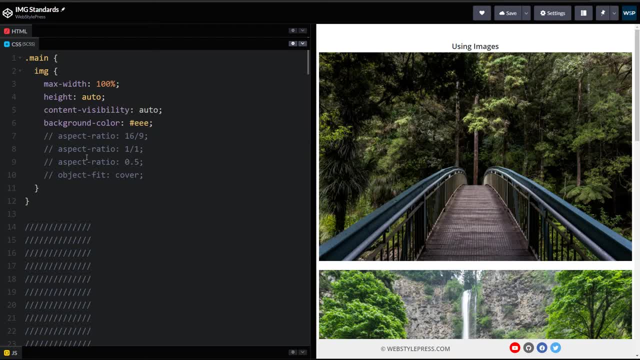 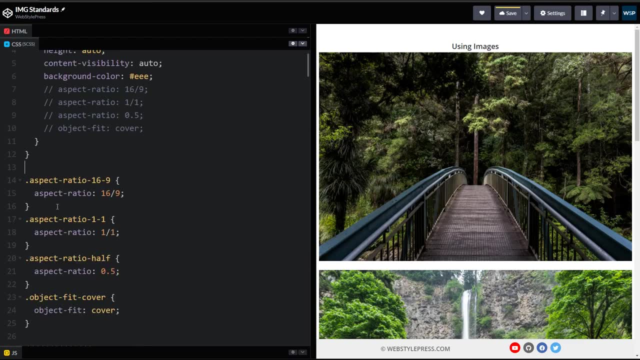 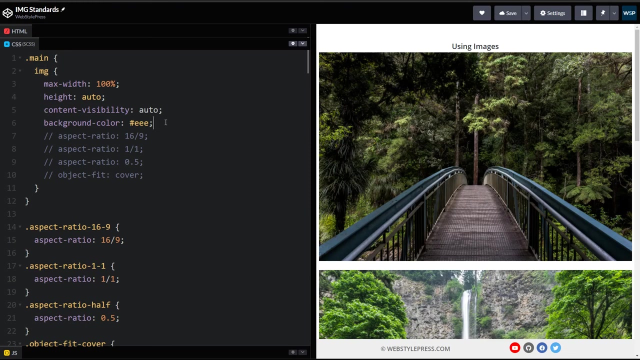 as it is not. you can create separate classes for these, you can have separate classes for aspect ratio and you can use these for individual images, depending on their size and orientation when needed. so important thing is this: content: visibility: auto and background. color: light gray. you can choose any other color as you like, so I am adding these two and then I have these two. 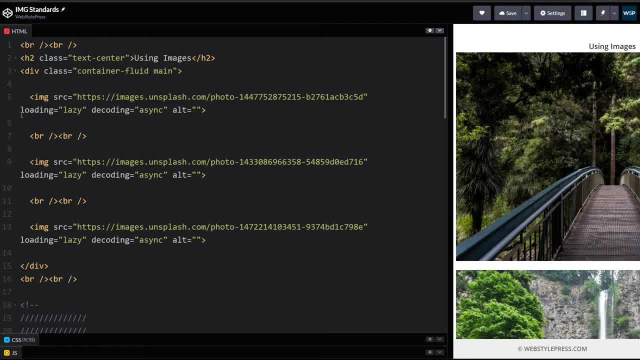 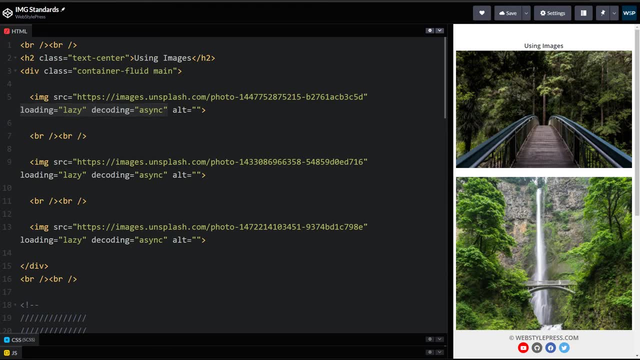 attributes for image loading lazy and decoding async. there are many other things that go along with these image optimizations, for example, using multiple images as source for different screens and more. I will explain those in other video, so stay tuned for that. ok, like, share, subscribe and I will see you in the next video.